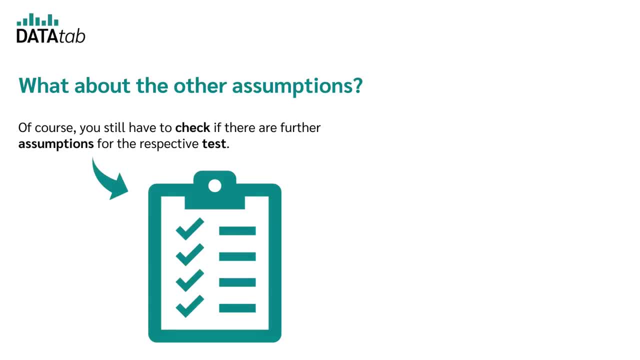 Of course you still have to check if there are further assumptions for the respective tests, But in general there are less assumptions for non-parametric tests than for parametric tests. So why then do we need parametric tests? Parametric tests are generally more powerful than non-parametric tests. 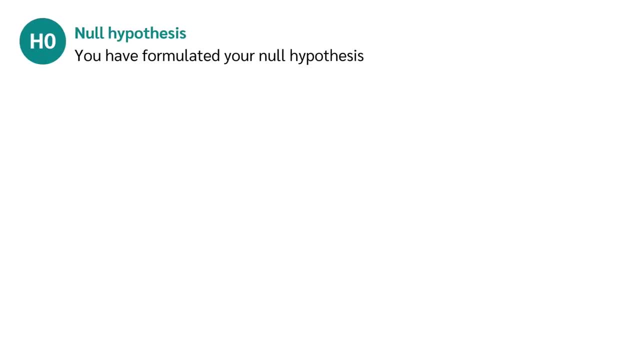 What does that mean? Let's say you have formulated your null hypothesis, which is, for example, the salary of men and women does not differ. Whether the null hypothesis is rejected depends on the following things: On the difference in the salary And also on the sample size. 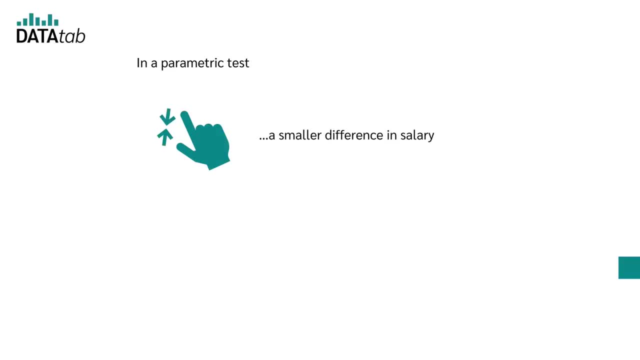 In a parametric test, a smaller difference in the salary or a smaller sample is usually sufficient to reject the null hypothesis. So, if possible, always use parametric tests. And now there are still two open topics. First I'll show you what the most common 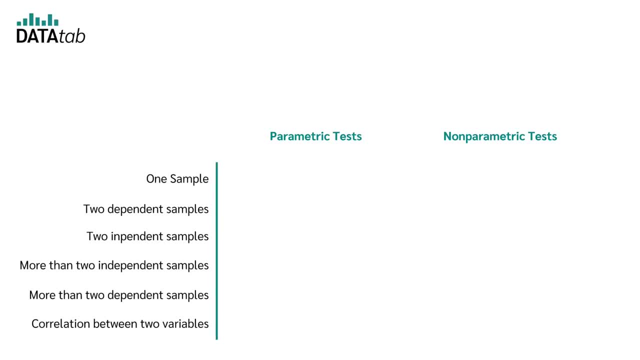 parametric and non-parametric tests are, And then I will explain to you how you can easily calculate these tests online with DataTab. Usually, for the most common parametric tests, there is always a non-parametric counterpart If you only have one sample. the parametric test is the simple t-test. 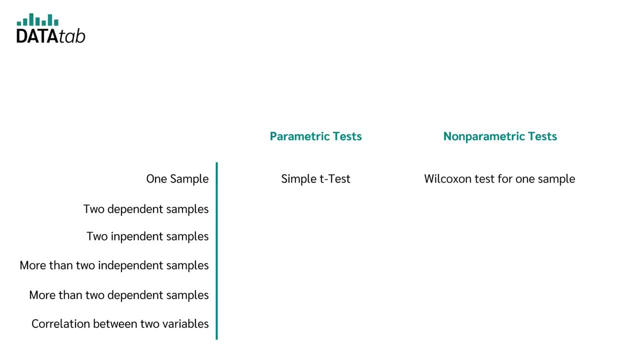 and the non-parametric test is the non-parametric test is the Wilcoxon test for one sample. If you have two dependent samples, on one side it is the paired t-test and on the other side it is the Wilcoxon test. 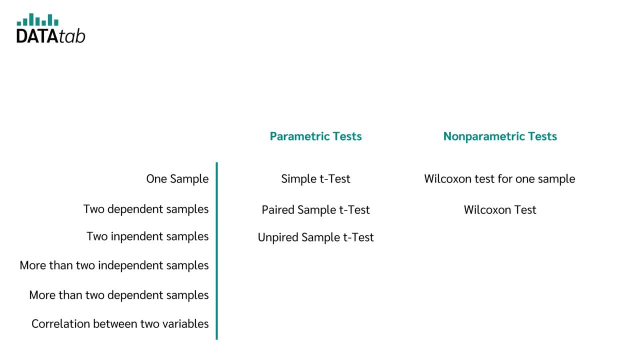 If we look at independent samples, it's the unpaired t-test and the Mann-Whitney U test. If you don't know exactly what dependent and independent samples are, just watch my video about it. you can find the link in the video description below. 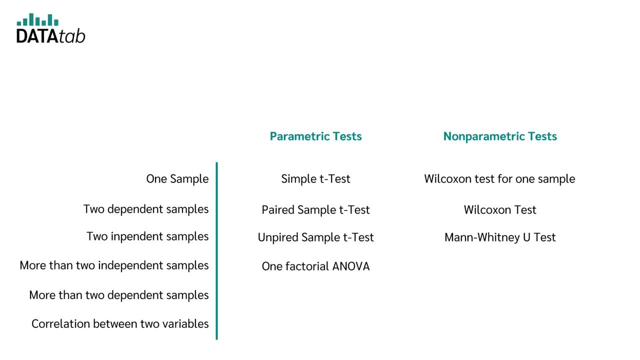 If you have more than two independent samples, you use the analysis of variance or the Kruskal-Wallis test. And finally, if you have more than two dependent groups, you use the ANOVA with repeated measures or the Friedman test If you want to calculate the correlation between two variables. 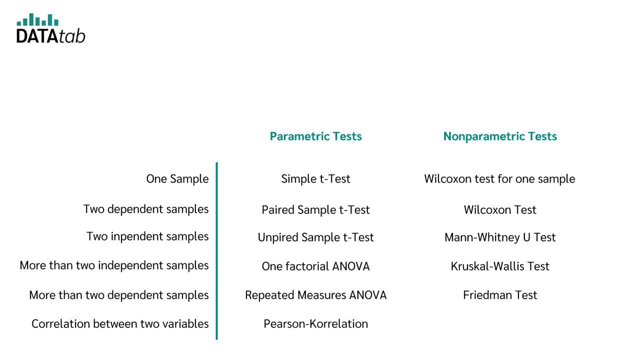 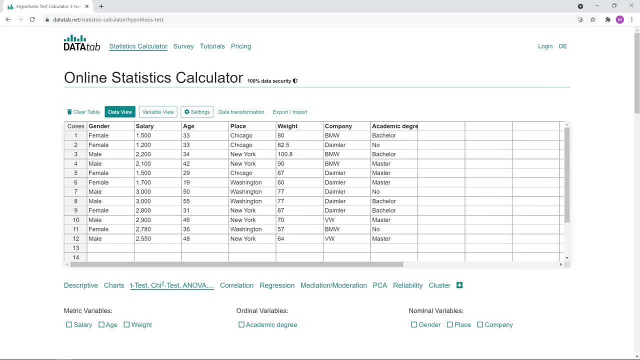 you can use either the Pearson correlation or the Spearman correlation. You can find the link to this overview in the video description. If you want to analyze your data by using data tab, you just visit datadepnet and you click on the statistics calculator. Then you can copy your data into this table. 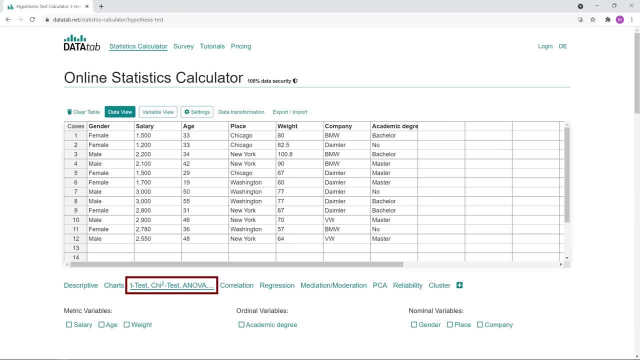 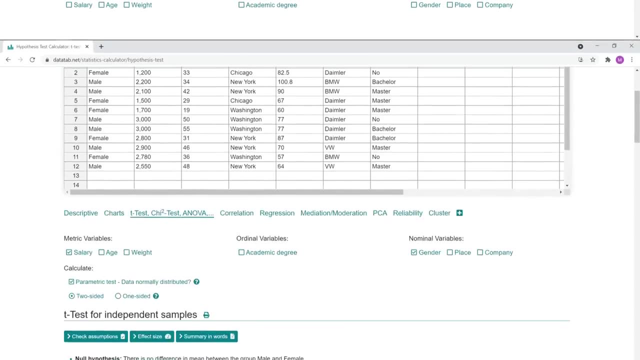 and click on this tab which says t-test, g-square test, ANOVA and so on. Let's say that you want to calculate the correlation between two different samples. If you want to calculate the correlation between two different samples, you just click on the statistics calculator. 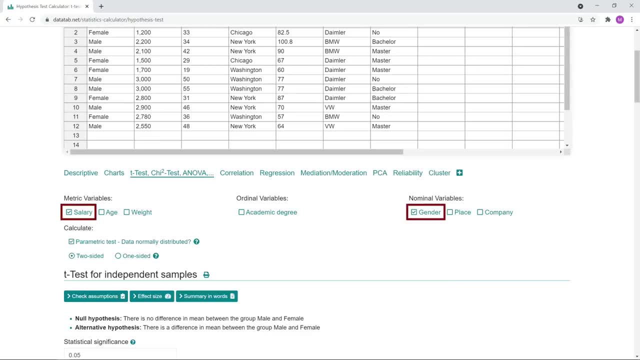 You choose salary as a metric variable and as a nominal variable- gender, Then automatically a t-test for independent samples is calculated, which is a parametric test. If you want, you can also click here. then a non-parametric test will be calculated. 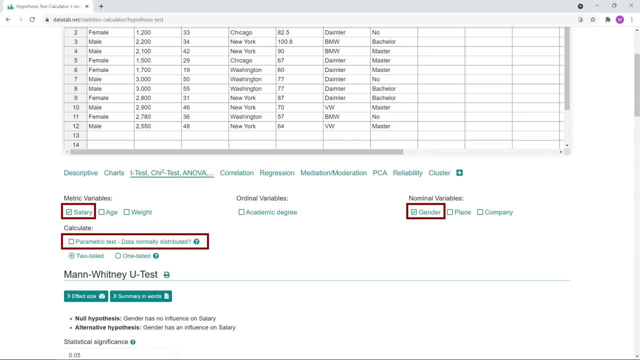 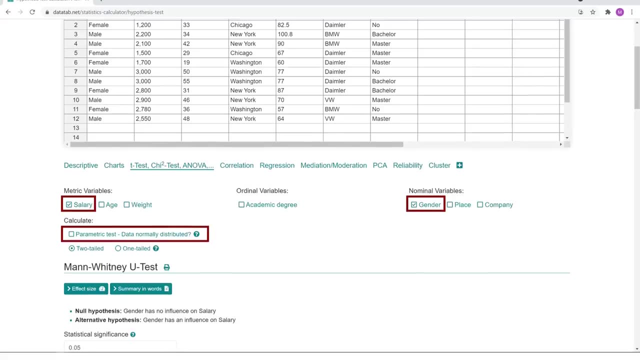 Then you can see that the Mann-Whitney U test is calculated, which is the non-parametric test. Then you can see that the Mann-Whitney U test is calculated, which is the non-parametric test. I hope you liked this video and thank you for watching.